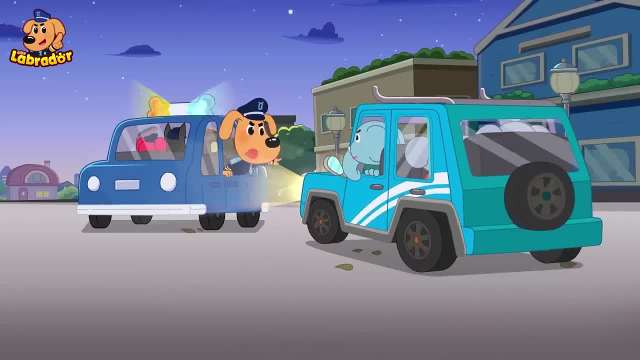 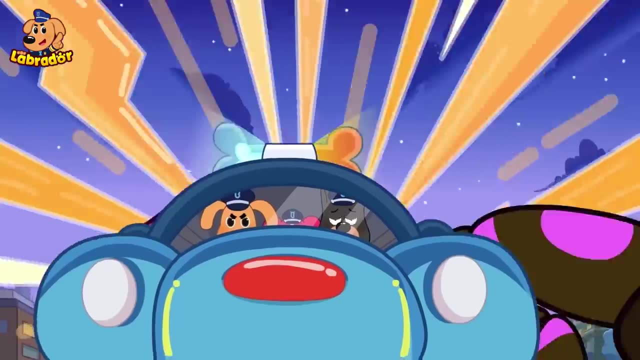 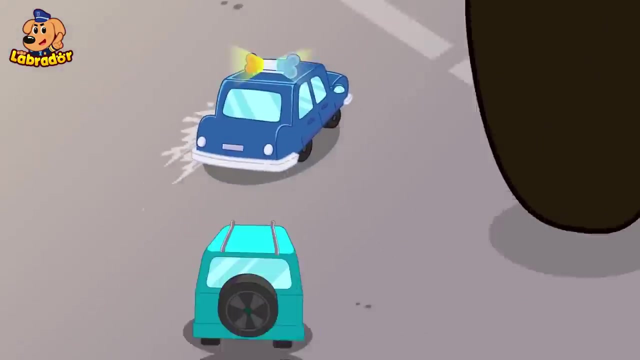 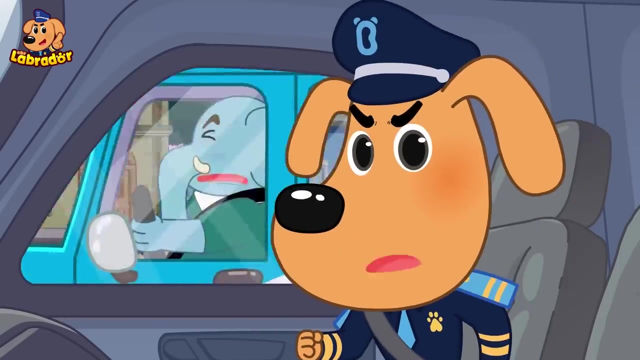 Mr Elephant, let's get out of here. It's catching up with us. Why is it chasing us? Let's make it stop, Let's go. Huh Huh, It might be attracted by the car's lights. Turn them off now. 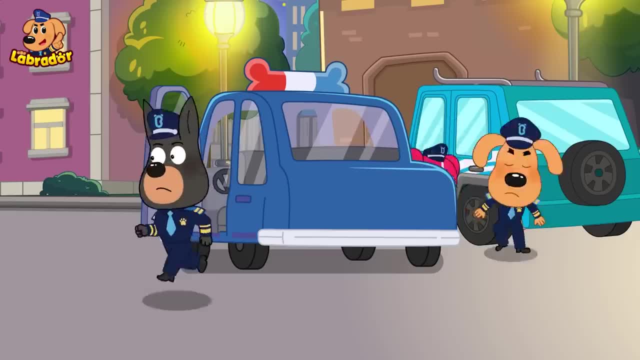 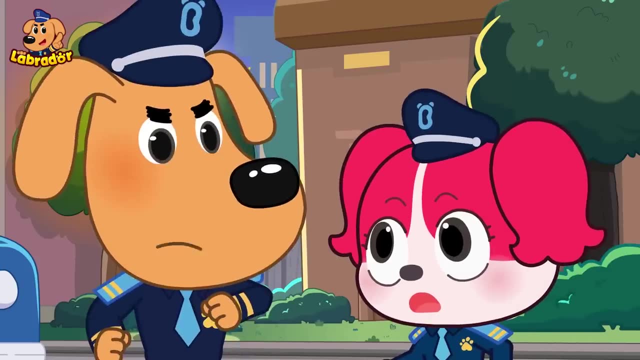 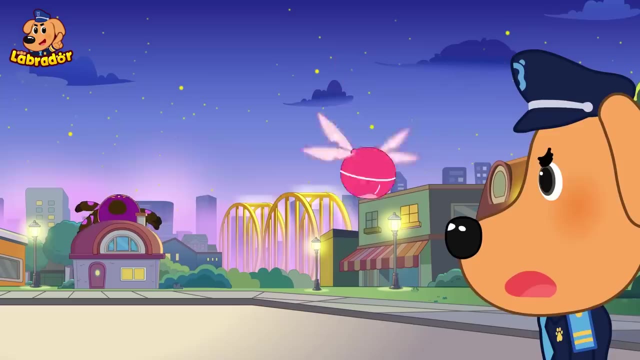 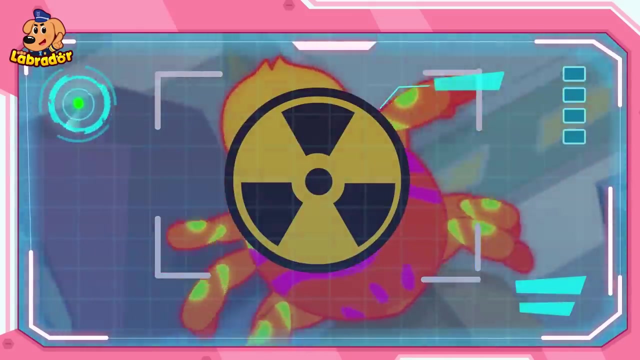 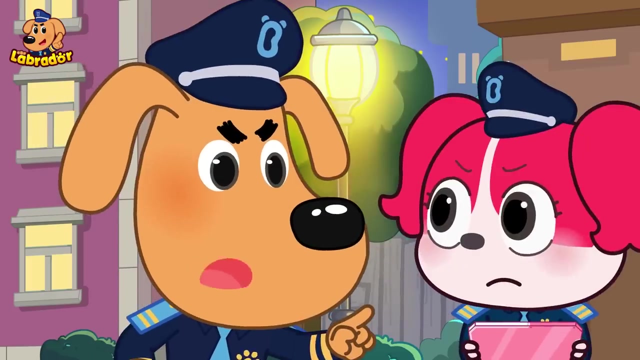 Phew, It finally went away. That was so scary. There must be something wrong with that spider Papillon. check it out. Huh, Activate flying eyes, Warning, Warning: Nuclear radiation detected. What's nuclear radiation? Nuclear radiation is a special type of energy. 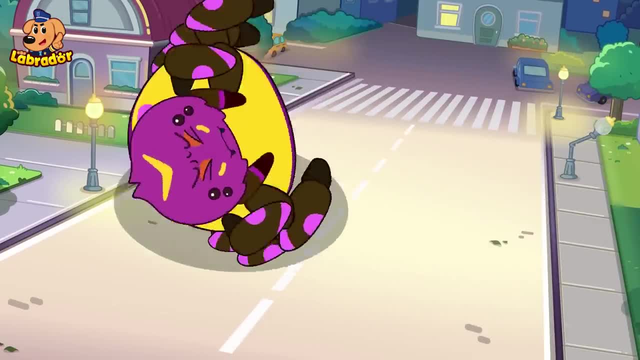 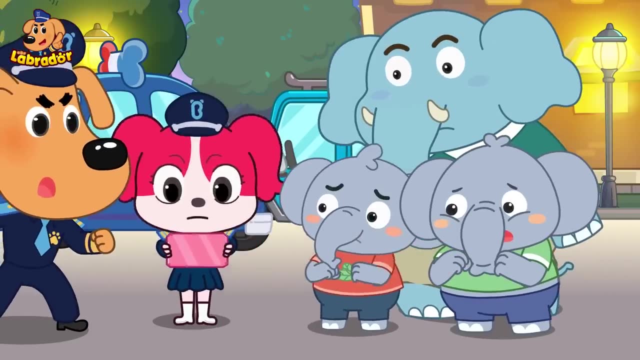 If living things are exposed to it, they might turn into something different and then disappear. They could even lose their lives. Oh no, That's so scary. The spider looks like it's in pain. Look, The radiation's coming from this chain. 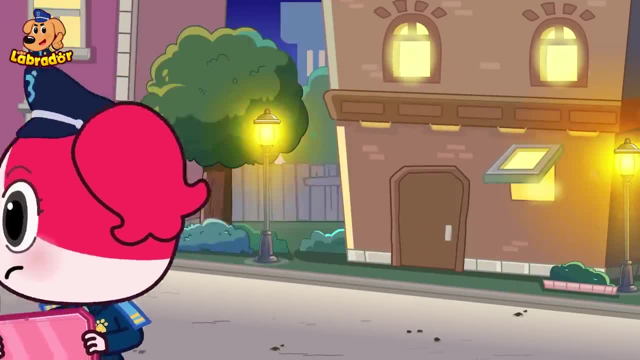 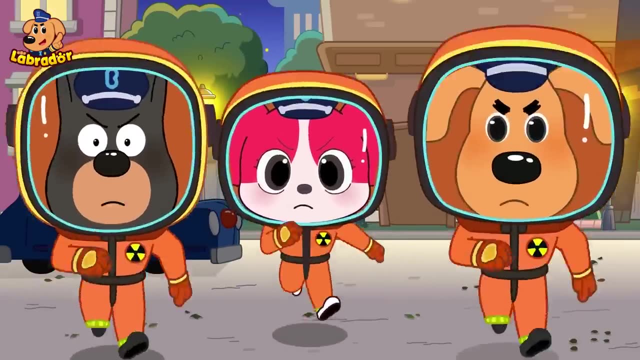 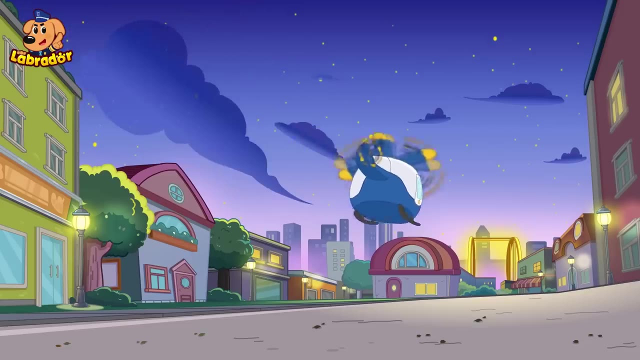 We have to remove it now and shield it. We're ready to go. Let's go. You can do it, Papillon. Come on, I can't. I don't think we can make it. We have to get the chain. 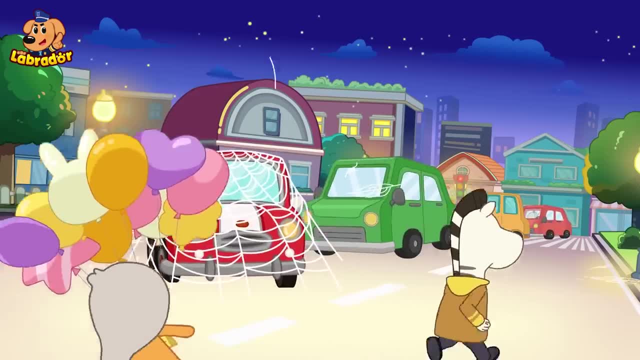 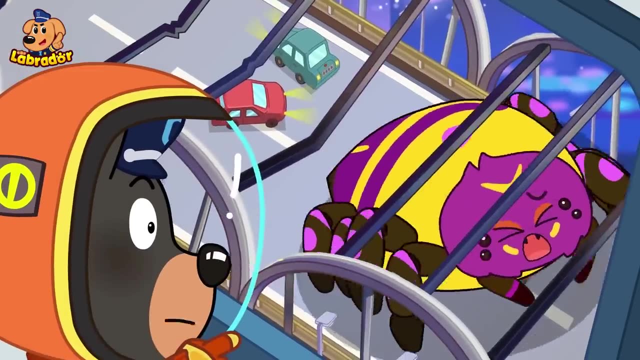 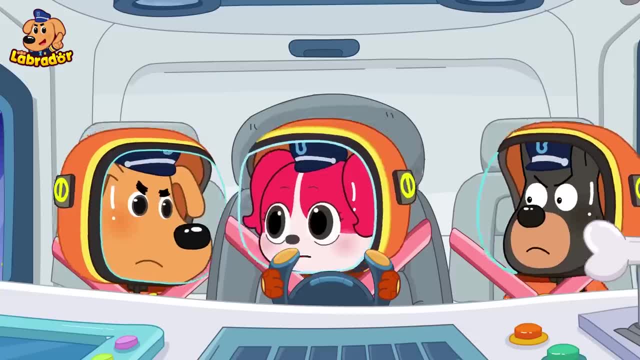 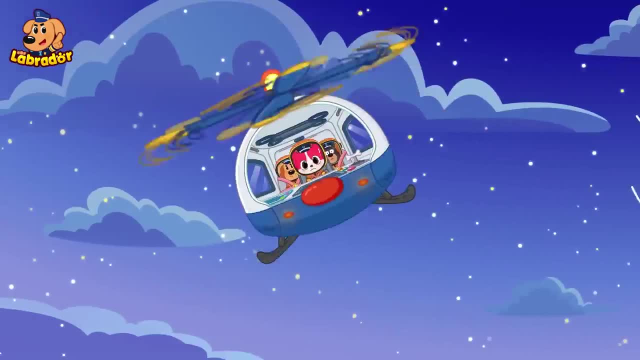 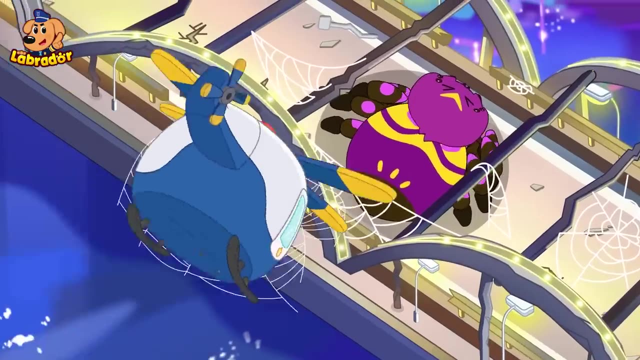 It's a big spider Run. Ah. Look, The spider got even bigger. Papillon, get close to it. Toby, let's go get the chain, Got it? Hmph, Ah, Ah, Oh, no, We're stuck.